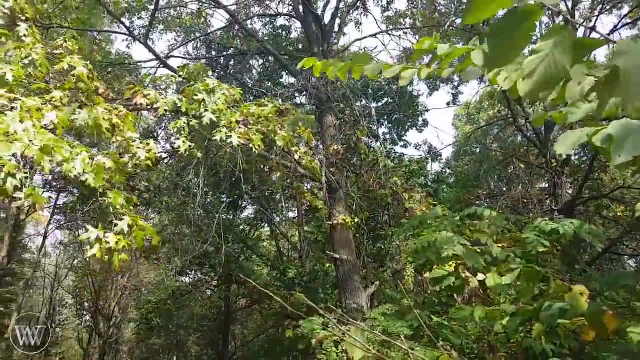 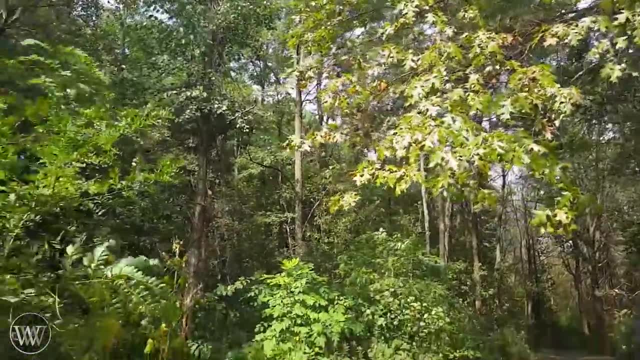 to come out and identify trees. It is not winter yet. The leaves are still fairly green, but starting to change, Some of them starting to fall. There's fruit on the trees, fruit on the ground, and we can walk around and quickly and easily identify them. Now, one I see right here is red oak You. 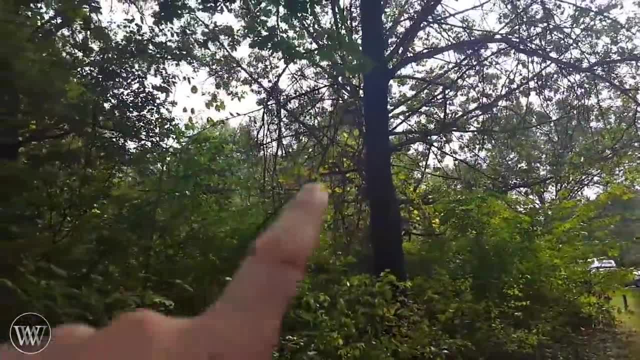 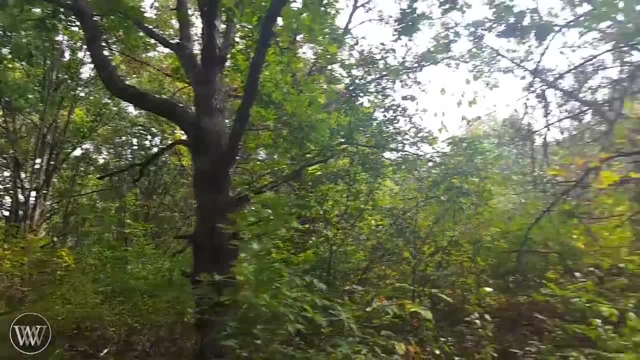 can see how these have very plump leaves. You can see how these have very plump leaves, Pointy leaves. So here I have two trees right next to each other- This one right here and this one right here- And they both are oak trees And they've become very, very obvious and easy to 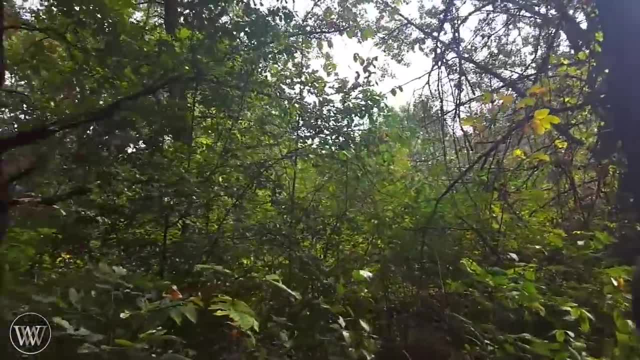 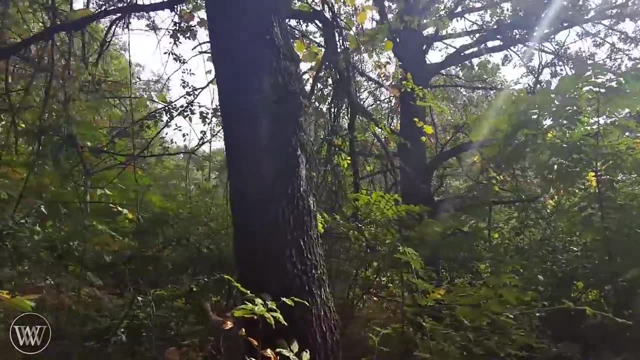 identify once you see them. The bark on these two is a little bit different. This one is older so it's a little more shaggy, kind of harder to identify, Whereas this one you have a little bit more of that standard oak. look, Let me take you over here and show you, basically one of the 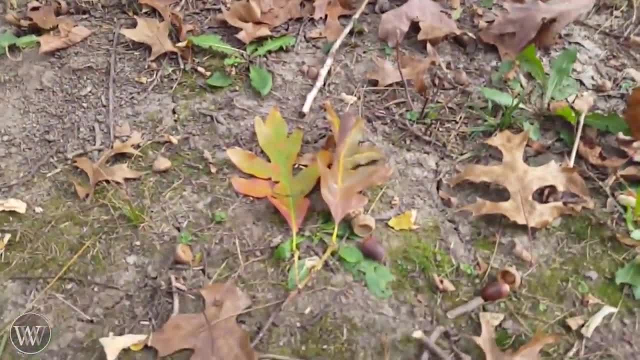 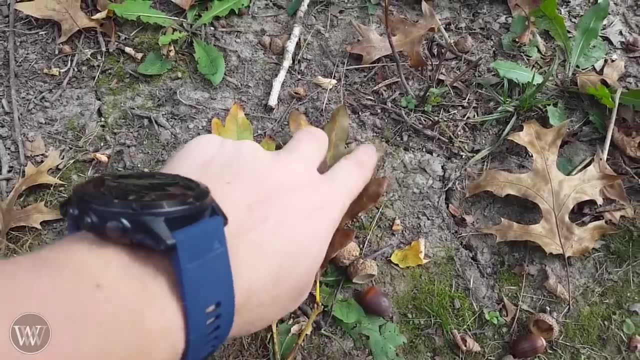 different types of oak trees. You get to identify their fruit and their leaves that are down on the ground. So here I have. this is from the first one over on my right and this is from the one on the left. You can see how all these have rounded ends on them. And then all these have these pointy ends. 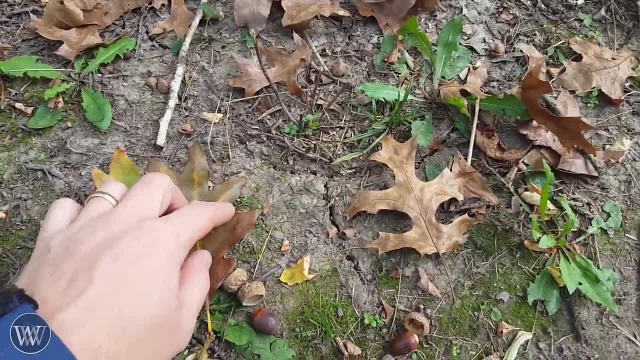 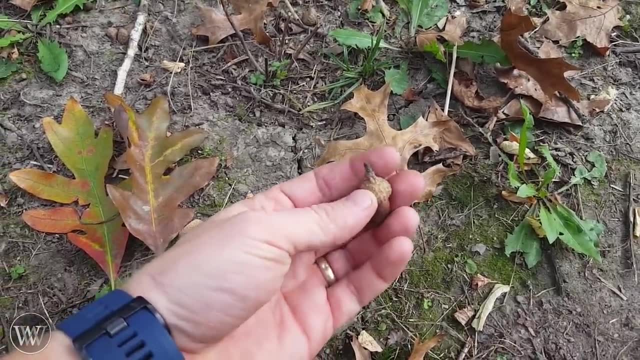 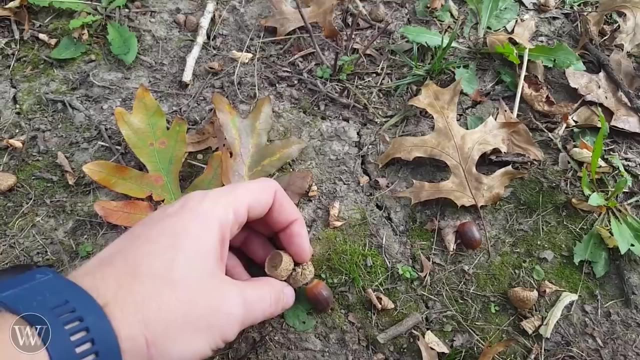 The pointy are from the red oak. Anything that's rounded are white oak. Also, you can look at the acorn, And the acorn from the red oak is usually a very smooth cap, not much identification to it, Or it's a very hairy cap And a lot of times the hair will actually hang down over, especially with 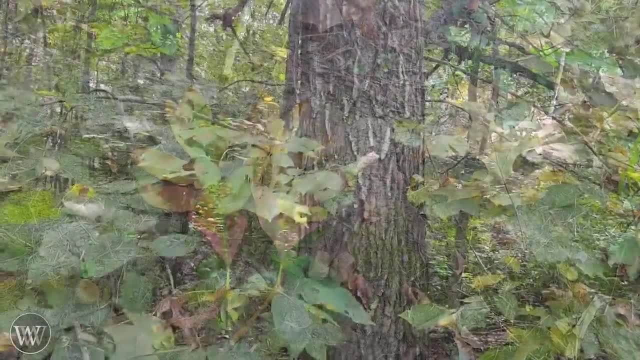 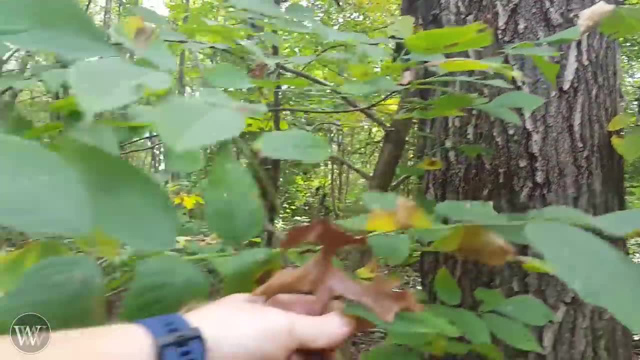 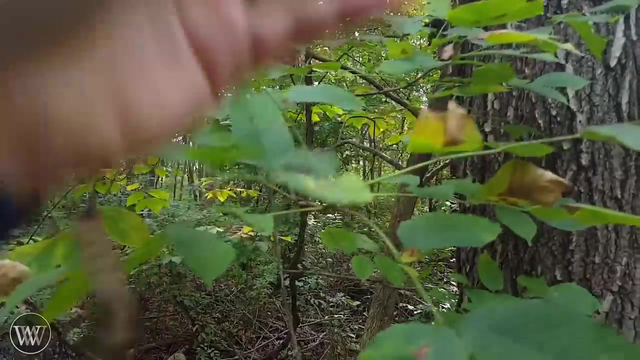 the bur oak and swamp oak. So let's go take a look at some others. Here's one that I like: This bark. it looks fairly similar to oak in many respects, But you'll see these leaves come off and it'll be the group of five leaves- Five or seven sometimes, Like on this one. you can see how they bunch out. 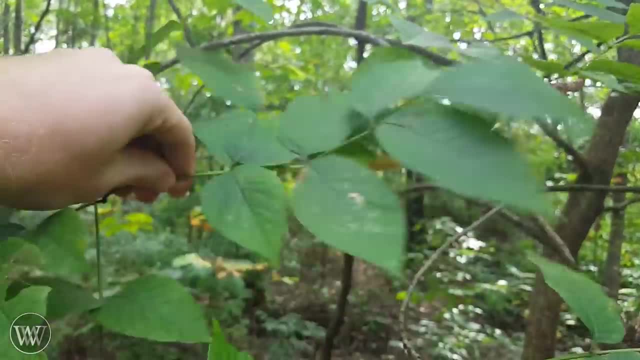 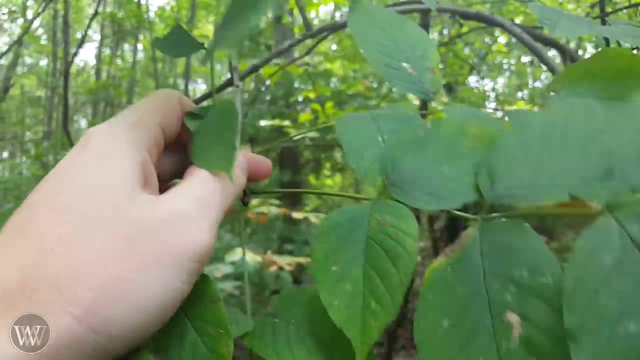 more, But here's the ash leaf, And they come in these whole series. You can see how they're clustered together. You might think that those are seven leaves, but this is actually one leaf that joins back at the stem. Ash is a very easy one to identify by the leaf, So here's one that. 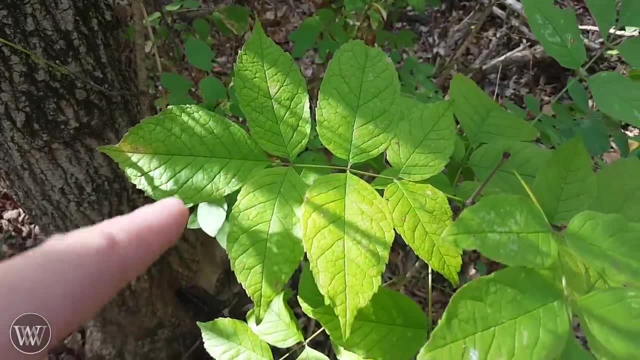 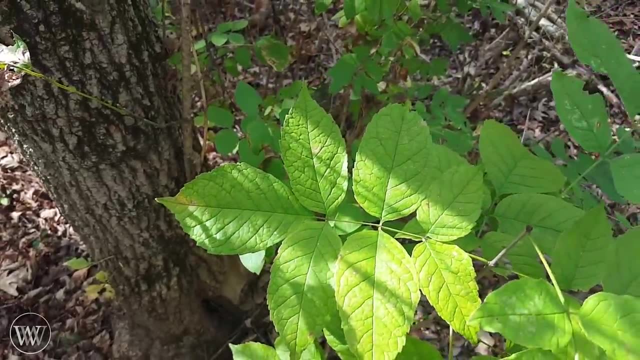 is a bit confusing. They may look like ash leaves that we just looked at. They're clustered together in seven. They're from a single bunch on the stem, But they're not ash. This is actually a type of maple. It is a box elder And after a little while you're going to get very used to identifying box. 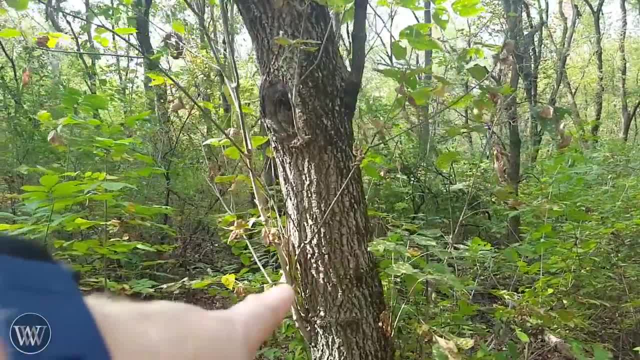 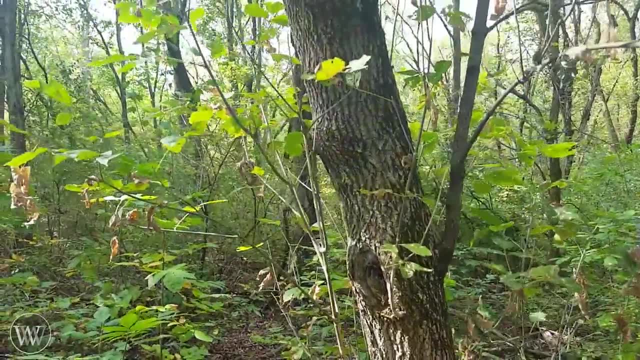 elder. by the branches and trees You'll often see this very distinctive bark and all of these little sprigs coming off everywhere. That's a very common representation of box elder. Very knotty, very twisty, It's not a hard maple. 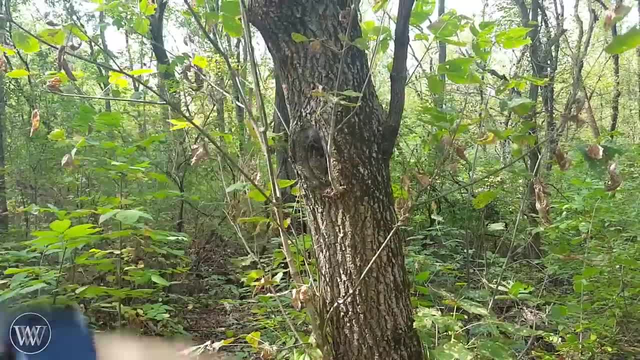 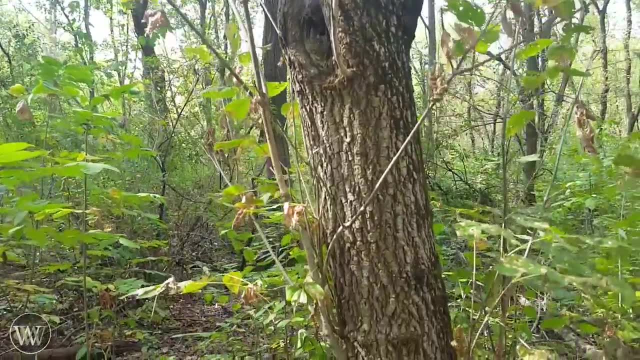 but it is a really nice maple with a lot of color in it. Sometimes you get a red flame through it. A very beautiful wood to work with and would make a great workbench in my mind. But yeah, box elder is a type of maple, often called ash leaf maple because the leaves well. 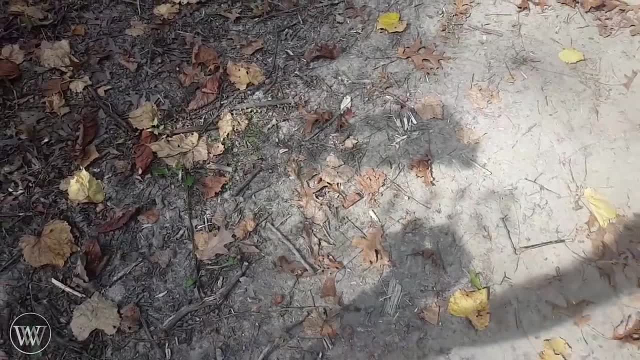 they kind of have a little bit of a dark color to them, But it's a type of maple that you can have a look of ash to them. Another thing I'm doing is I'm walking along and I'm looking for acorns, I'm looking for nuts, I'm looking for leaves And I'm starting to identify the leaves. 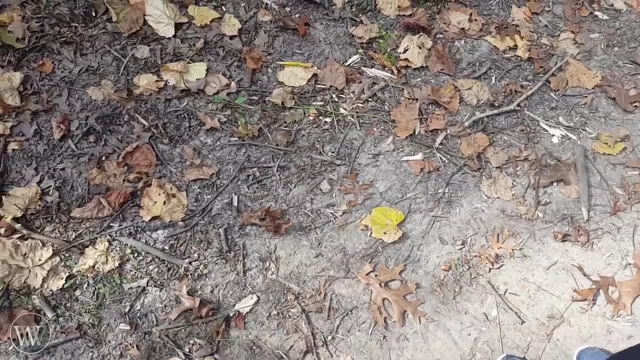 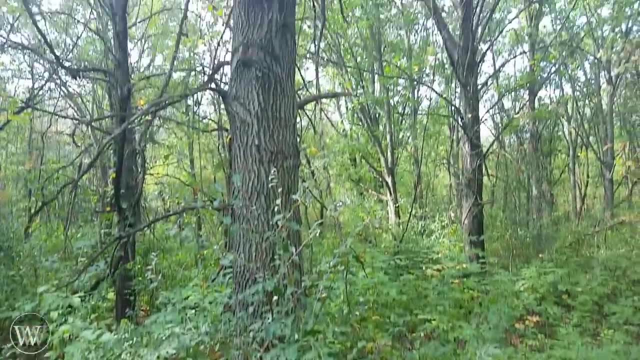 Like this one is a type of maple, That's a type of oak, And usually from the ground you can start to see where the leaves are And then you can look up into the trees and find out where are they. Is that? does that leaf look like the one I'm putting on the ground, Or does that leaf over there look? 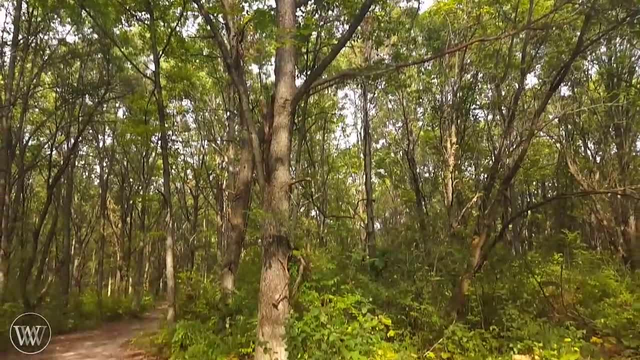 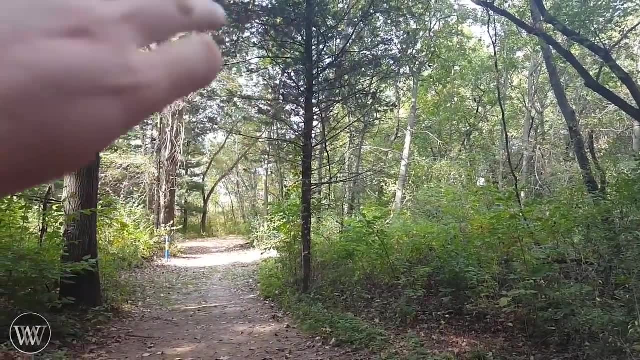 like the one on the ground, And then from there you can identify the bark on the tree And say, oh, I know what that is now. So we've been looking at hardwoods, but here you have a couple softwoods- This is a fir. And then you come back over here And this is a bark that you'll 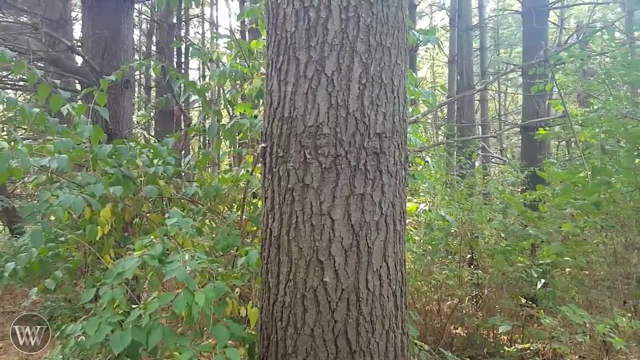 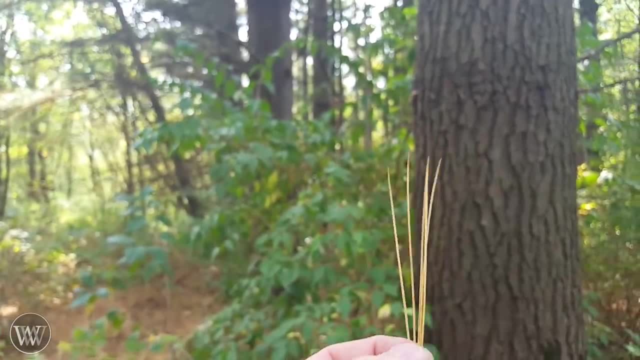 know quite a bit. This is a pine tree And I don't know as much about them because I don't use the wood as much and they don't interest me as much. But one of the things that's actually kind of fun for me are the needles, particularly from the white pine, because they're very long needles. 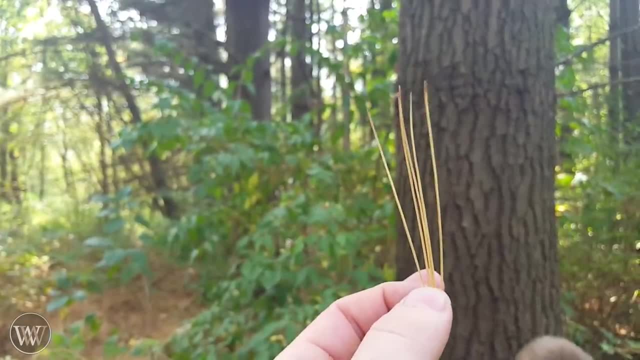 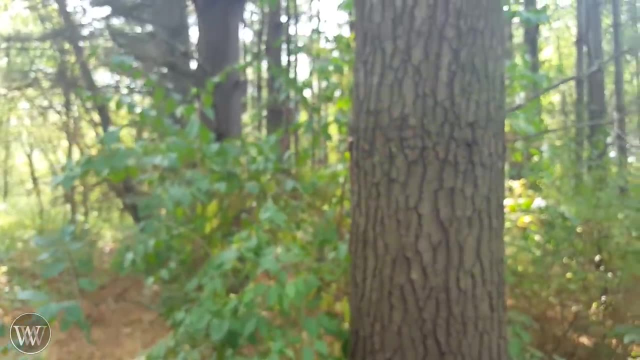 like that, And you'll find that they each have five sprigs, which is white, I-T-E. Five letters, five sprigs- A fairly easy one to identify, And one of my favorite pines. Okay, here's one that I really like. You'll find these heart-shaped leaves And they fall in great 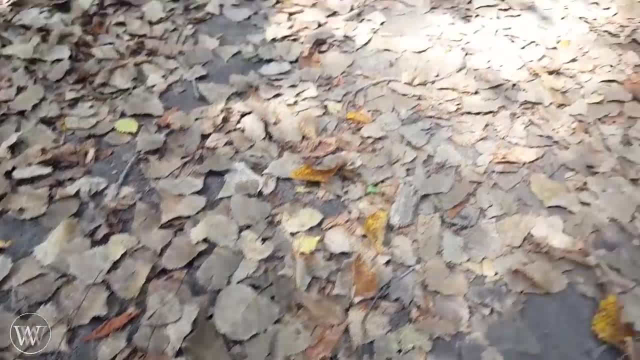 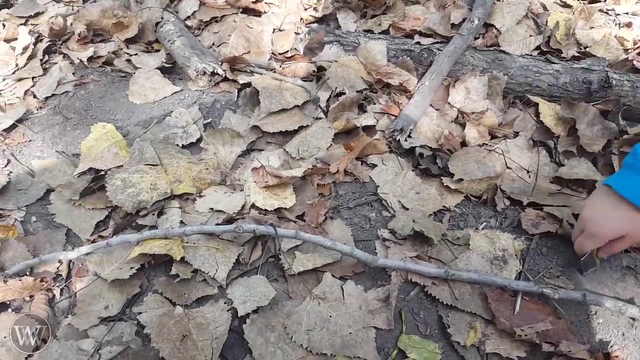 clumps. They don't change color that much And they just they clutter the ground. And you're also going to find these sticks that have a lot of nubs and nobbles on them, And these sticks are very telltale of cottonwood. So let's look around here. We found these all over the ground And 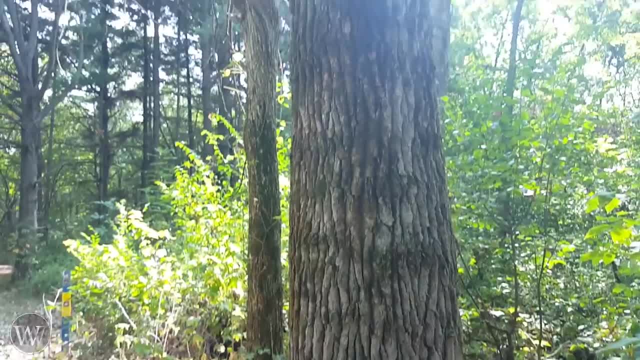 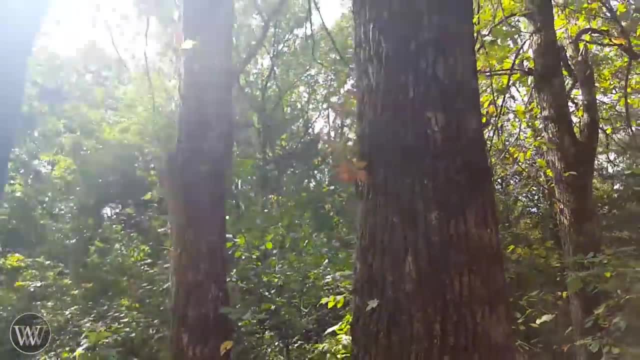 we're going to look around for usually a very large, large tree, And voila, there it is. This has a lot of bark twisting on it. They usually end up having a very, very straight, long trunk all the way up And you can see that they have a very large. 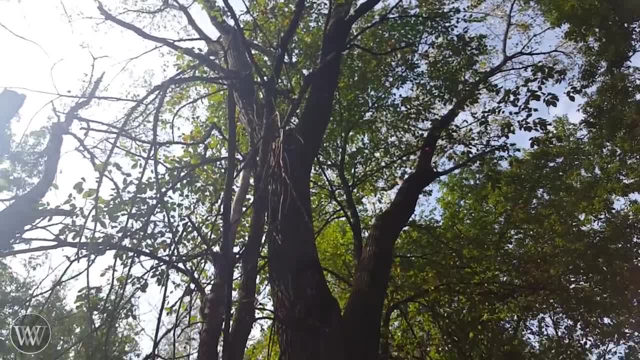 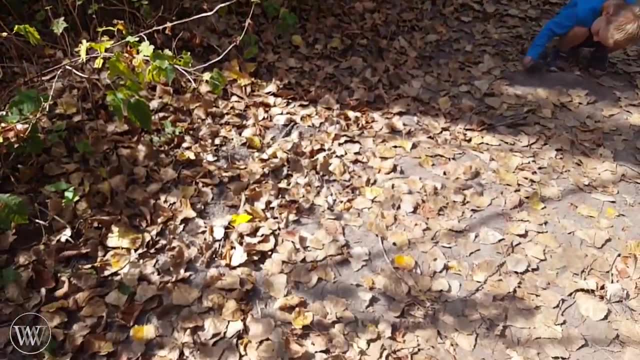 canopy. most of the time It's cottonwood. In early spring their seed will come floating down through the air in little tufts of cotton, But they are very, very easy to identify in the fall or any time by these leaves. Not too many trees have them, But they are very, very easy to identify in the fall or any time by these leaves. Not too many trees have them. 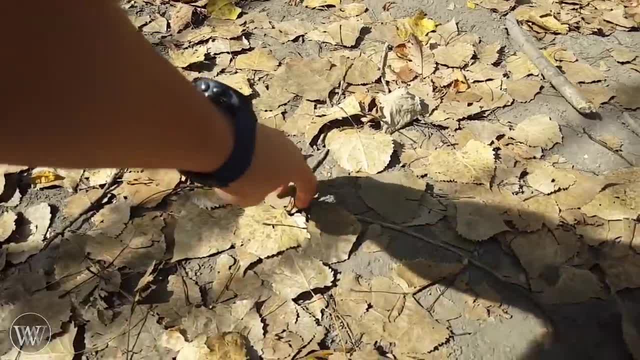 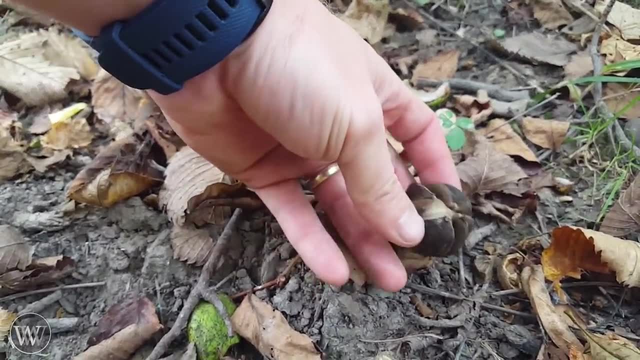 that leaves like these heart-shaped cottonwood leaves like that right there. So here's one of my favorites. You'll be walking along the path and you'll come across these nuts that are kind of split four ways. The husk falls off very easily And then you'll have these white nuts underneath. 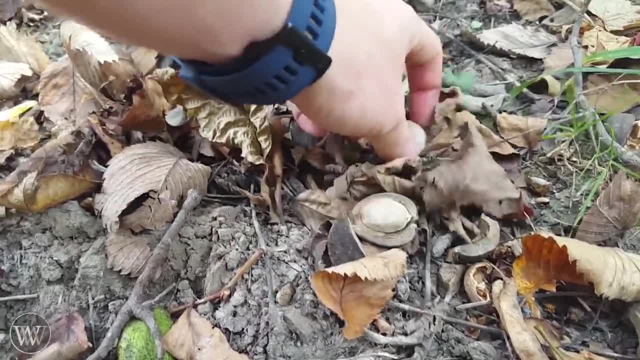 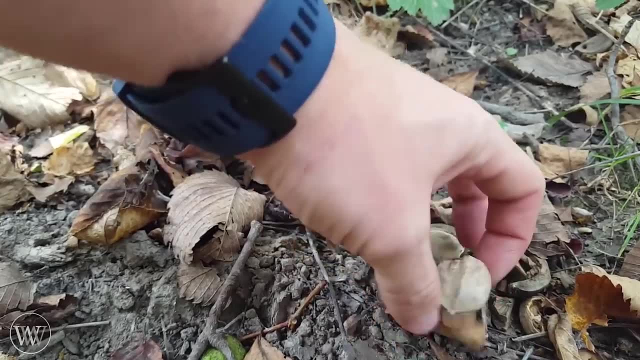 These are hickory nuts And hickory is one of my favorite woods. Beautiful, beautiful wood, extremely hard, great for axe handles and anything you don't want to break. Just gonna with it right there. This nut above is called d�� Disテs are not blowing. You actually have to be super. 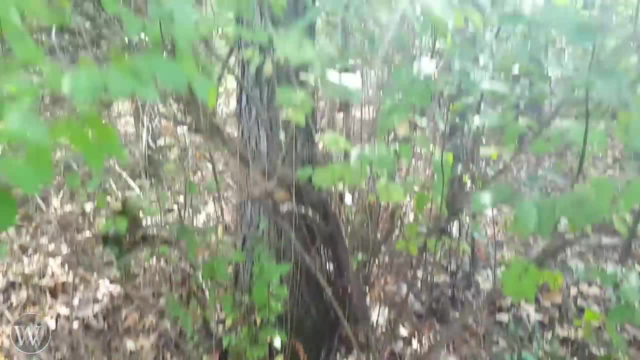 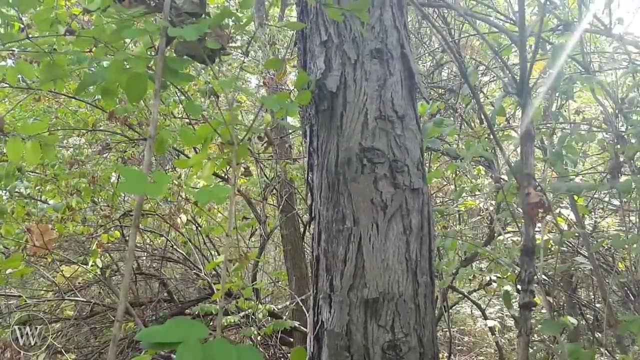 Just a great, great wood all around, but one of the cool things about it is the bark is very easy to identify. The bark here is actually this kind of shaggy thing that well, It just like these pieces will flake off, and this is a hickory tree. 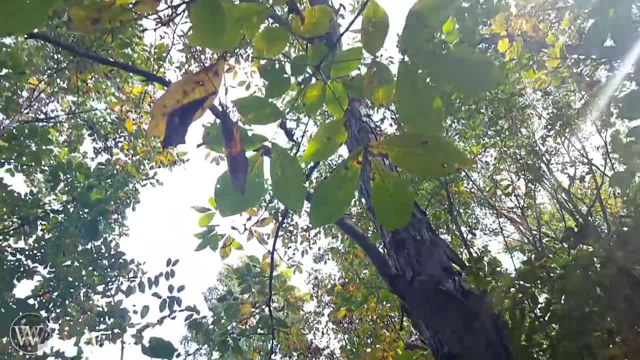 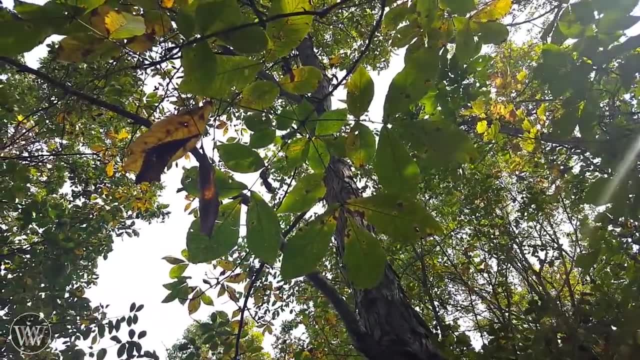 Now, if you go all the way up, then you get this almost. These things are huge and I'm trying to find one here on the ground, But they're about 12 inches long, so each one of those are about a foot long. They're huge, huge leaves, and you can see that each one of them has a cluster of three and then the stem coming off. 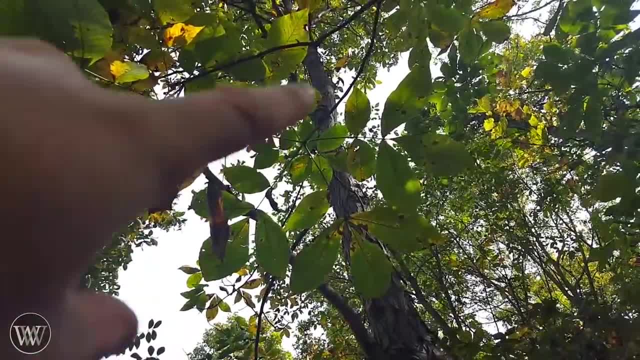 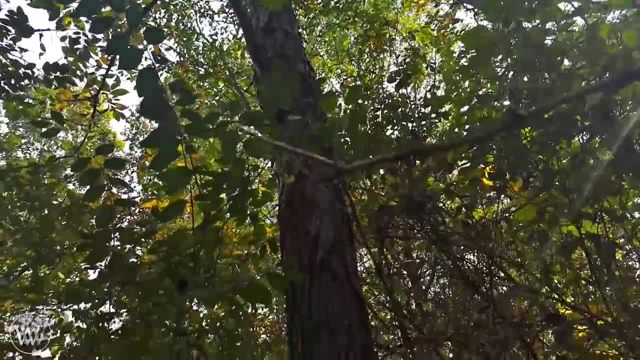 That's one leaf, is that cluster of three and the stem, and this one over here has five and one long stem. so they're a very beautiful tree, our great wood, to work with and a lot of fun when you identify them. plus, hickory nuts taste good and 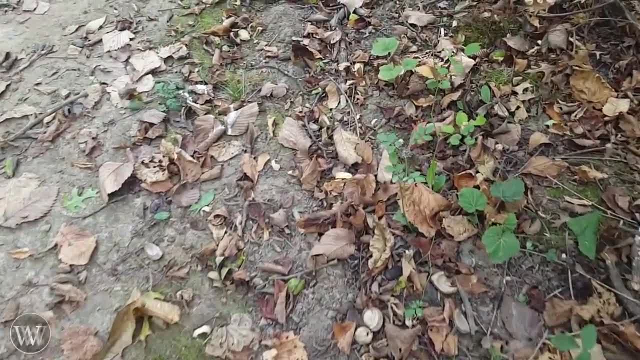 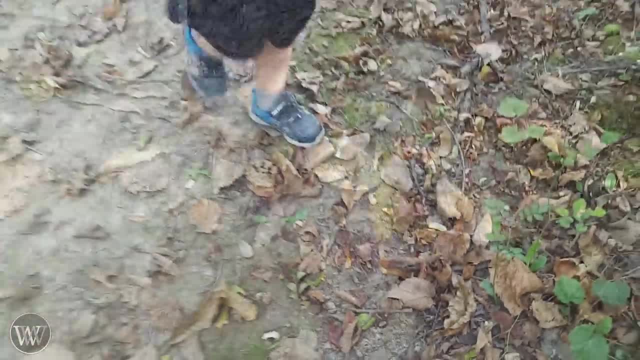 You can take those home and have fun with them. So yeah, I'm always finding these. I'm out running in the woods, You will stumble across them, and it's a very obvious problem That there's a hickory tree here, So here's another one. you're gonna find these oval Leafs quite often. 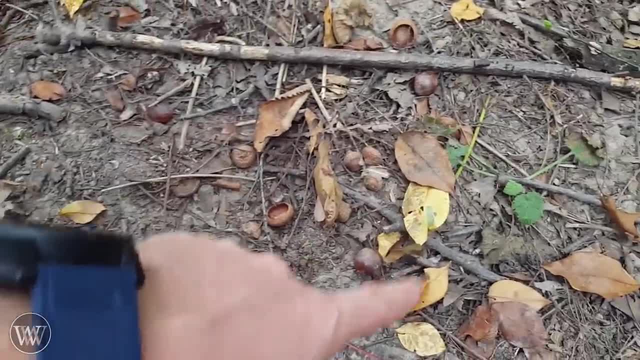 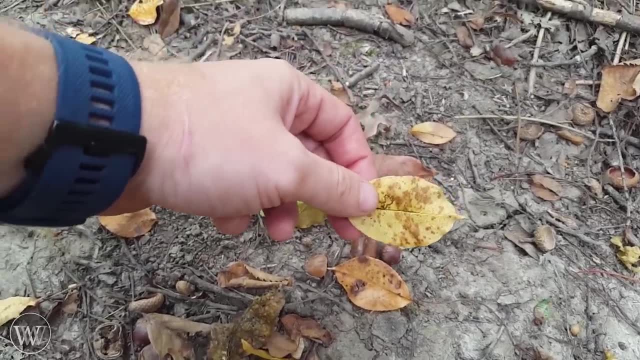 I'll be looking around and there's one here and one here and there's another one over here and here and here and there. They're fairly oval. some of them have a very fine sawtooth, like this one, so I have a very pronounced sawtooth. 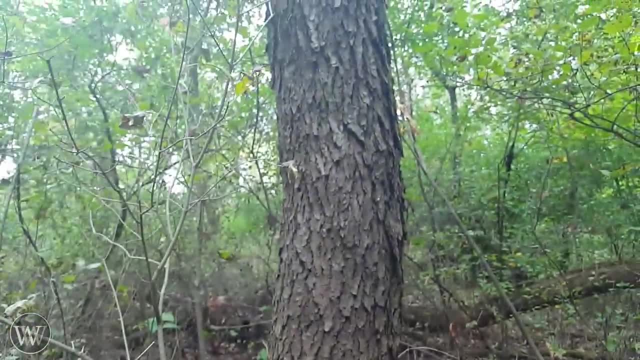 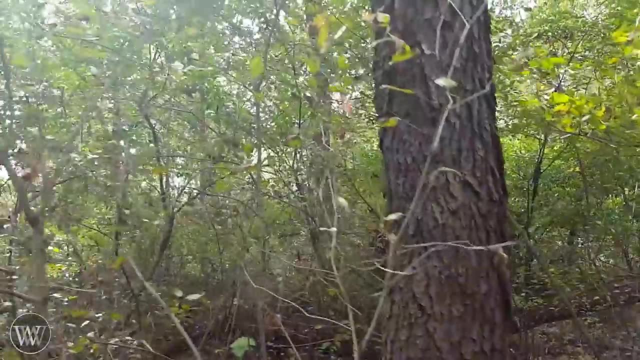 But then you also see these trees that, if you didn't know any better, you'd swear they were a pine tree. They kind of have that shaggy bark that you see very commonly in pine trees. That is actually a cherry tree, and a cherry is a fantastic hardwood for hand tools. 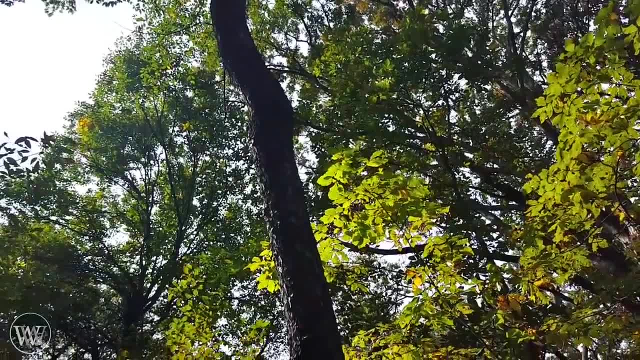 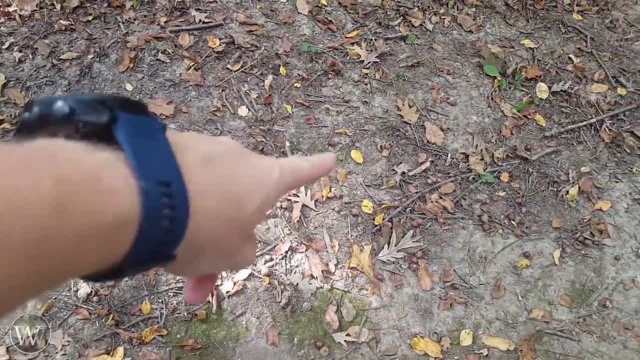 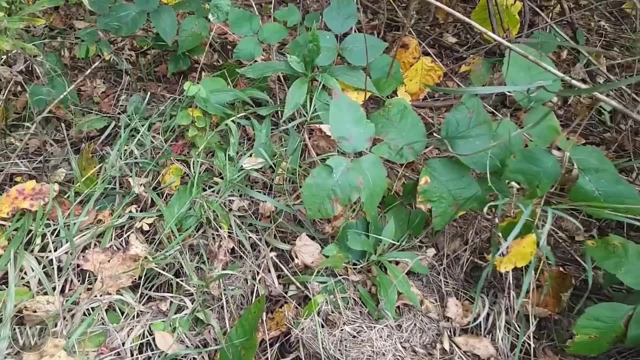 Just a beautiful, beautiful wood with a dark red color and one of my favorites. But yeah, you'll be looking along the floor and you'll come across all these little yellow, Tiny little leaves like that one there and that one there. there are cherry leaves. Now here's another one I want to identify. this isn't a tree, but if you're wandering around the woods, 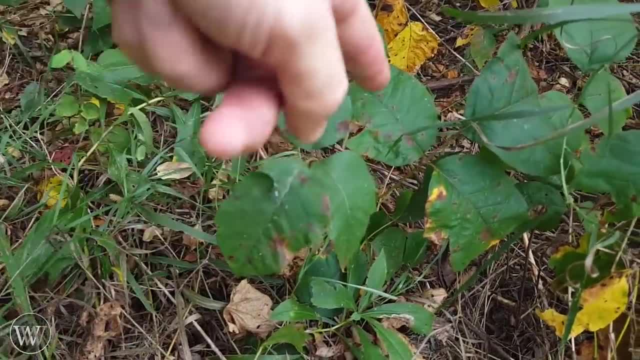 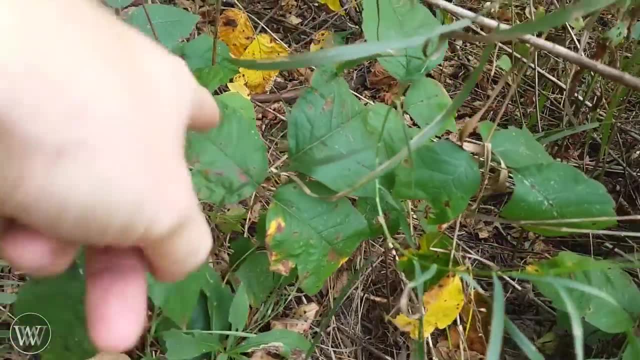 It's a good one to know, and you'll see these three leaves here, and Often they look like a mitten, and the one in the one in the middle will have a thumb on both sides. Where's the one on the outside will just have a thumb on the outside. 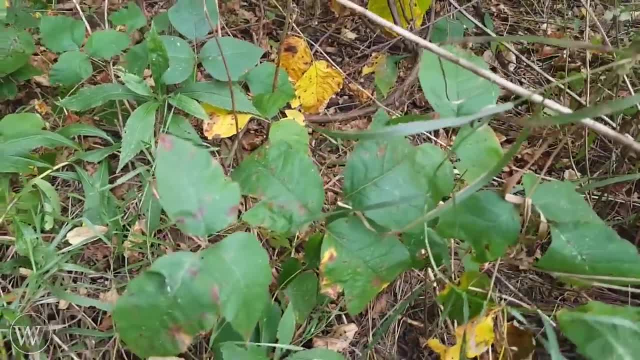 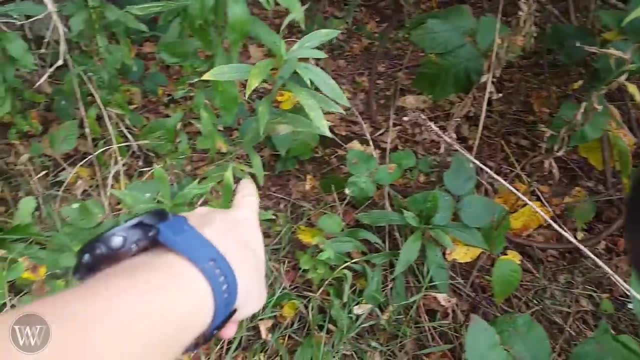 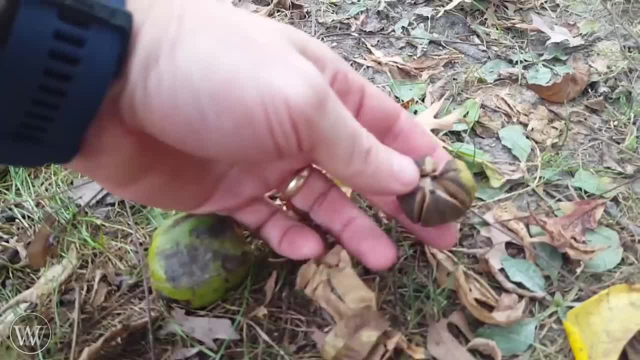 Okay, here's a fun one. So you're walking around the woods and you find this hickory nut, and a little while later you find this one. you think, Oh, is that a black walnut? No, it's a hickory nut. if you look closely, It's got this. 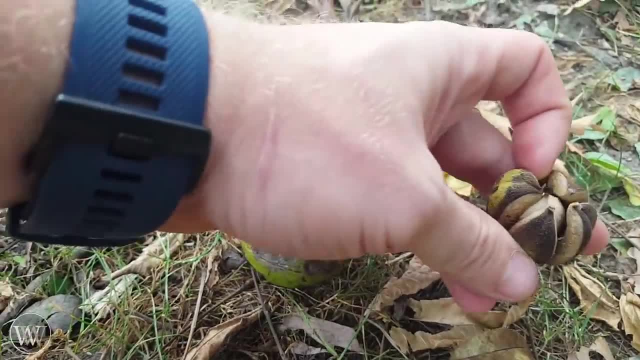 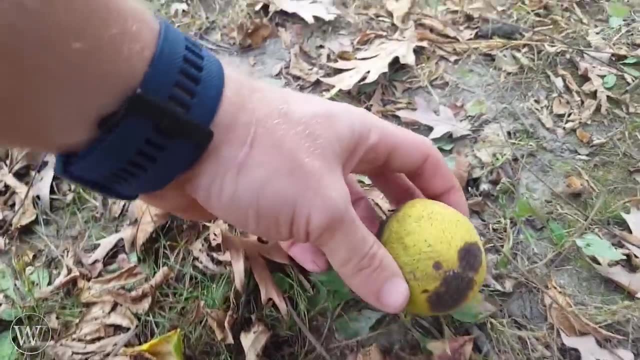 Cross-section at the top. It's just one that hasn't turned black yet, hadn't gotten soft, so you can pop off the husk. a Walnut- though a black walnut- looks like this, a little smaller than a baseball. when they come down, They're green and they slowly turn black and then eventually the black all falls off. 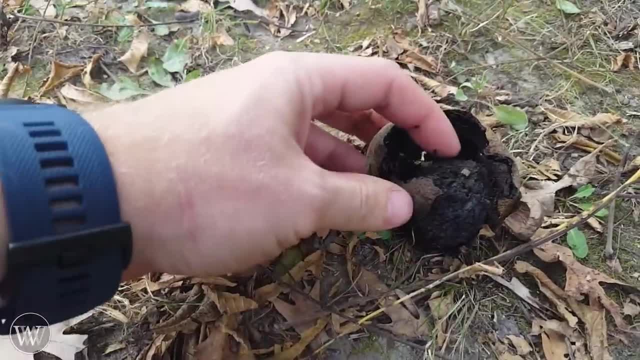 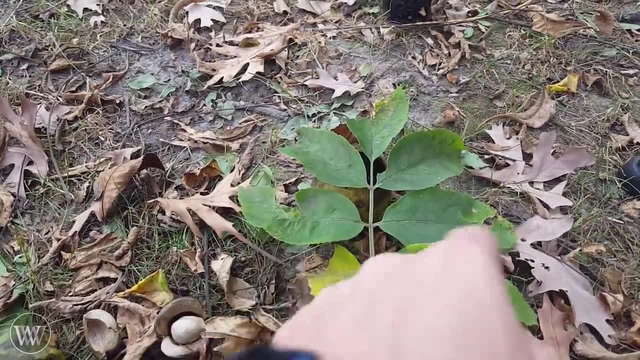 And you'll see this traditional or like a walnut inside the leaves Look kind of like an ash leaf and that they're all one big piece and they have these sprigs that come off, But they're very hairy, They're fuzzy and they have this like characteristic to them. 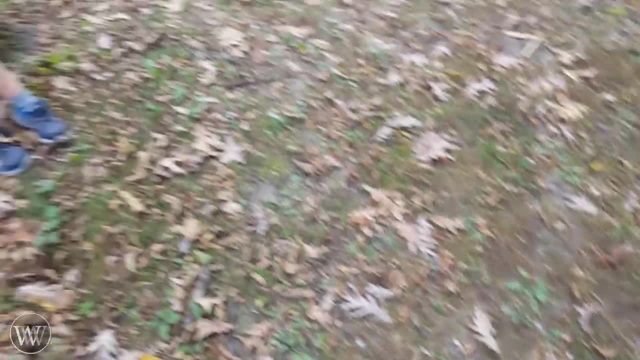 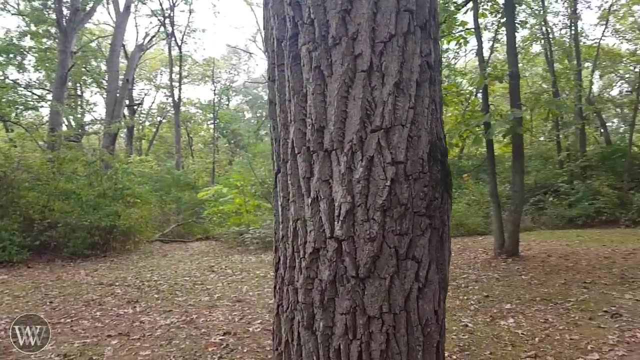 The center of the stick is very pithy and then the bark is very easy to identify. It comes like this: you see this, this crisscross X shape on the bark, and that is very Characteristic of a walnut tree, and so you know this right behind the bark. 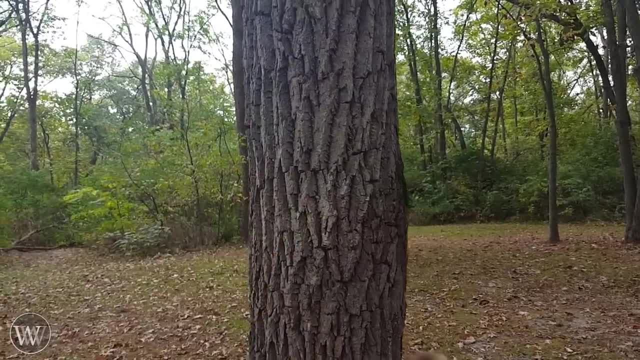 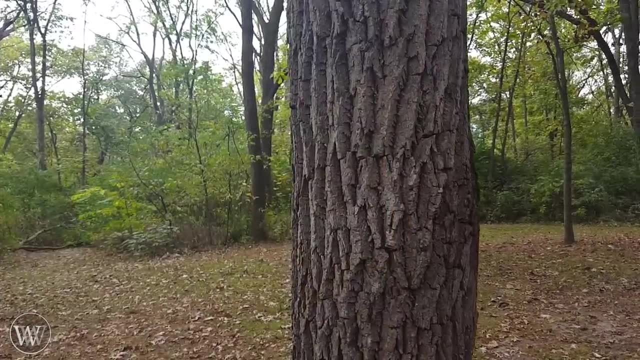 There's a bit of a white wood, the sapwood, and then inside of it You're gonna have that very, very dark Walnut wood and then the very core. you're gonna be almost this almost empty Core running all the way up the middle in the heart of the tree. 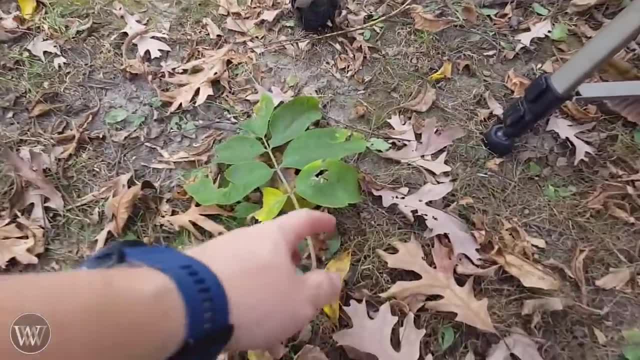 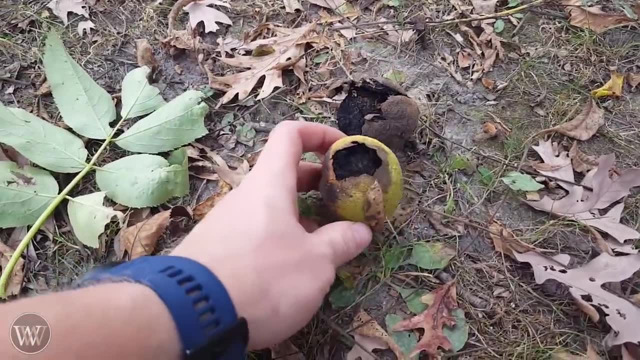 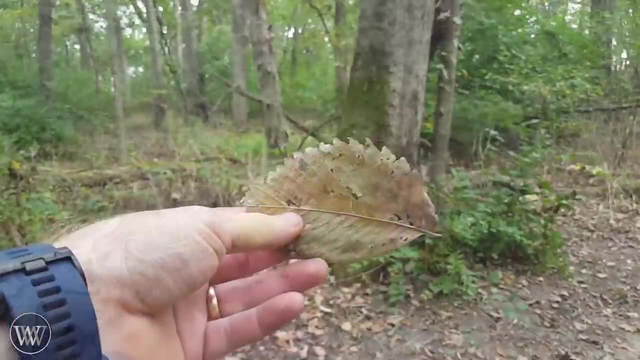 So yeah, when you're running through the woods, You're gonna come across these nuts and they become a problem for stepping on. because you step on them, you roll. but this is black walnut and Once you start to identify it, you'll be very, very happy you did, because everybody likes black walnut now. 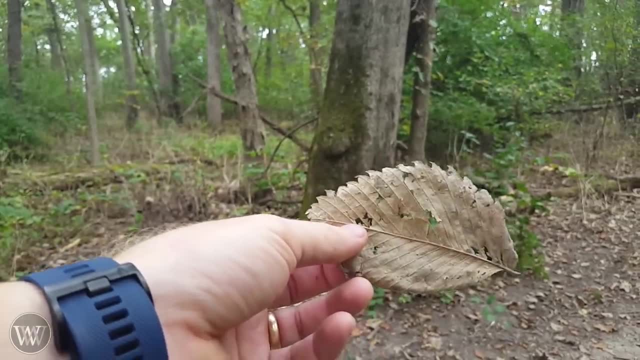 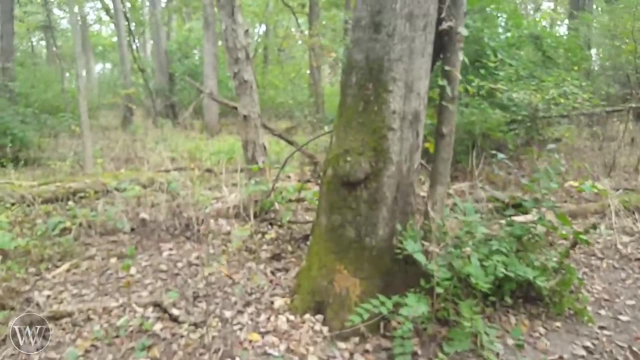 Here's one that I should know. it has a sawtooth leaf and all the spines come back to the central point As opposed to all coming to the base. They all come back to the main spine And I'm seeing this tree quite often. I've seen these leaves a lot. 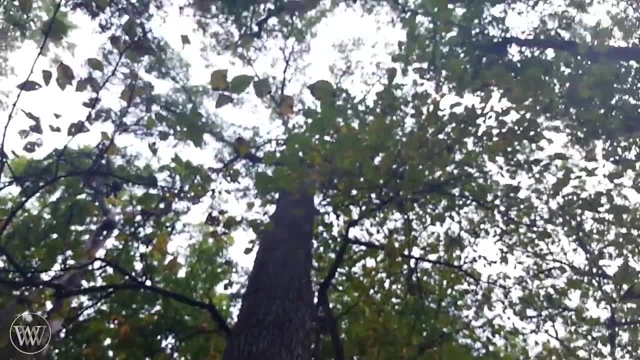 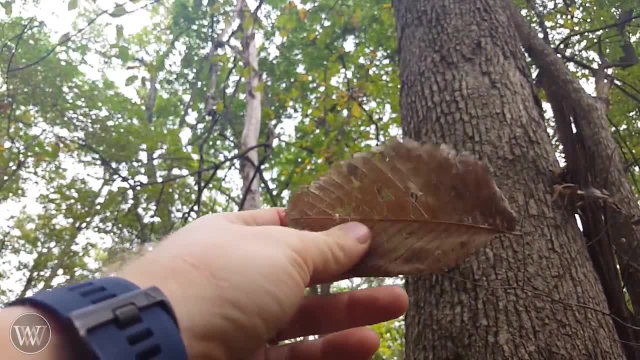 They are all over the place and you can get a closer look at what the canopy looks like. Well, kind of okay, But these leaves are just covering the trees and they're all over the ground. So when I get back to my house I'll show you how I look it up and identify the tree. 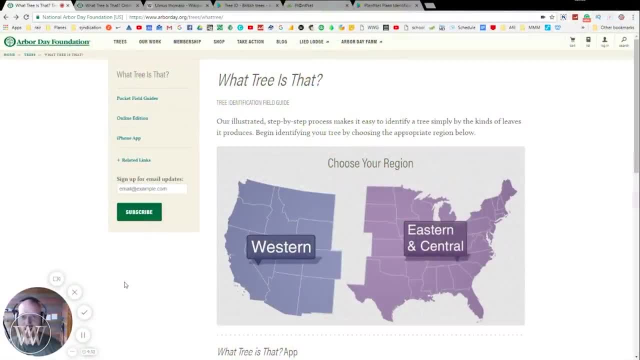 So now let me take you to a few sites and apps that I use to help me find What is this plant, What is this tree? and my first and foremost is the Arbor Day Foundation, arbor day dot org. and I'll leave a link to all of these apps and websites down below so you can go and look at. 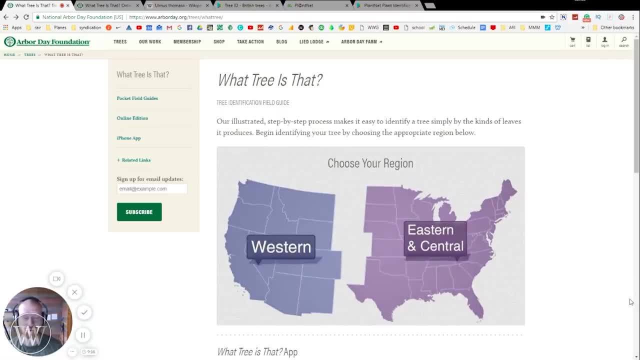 That and this one is very good, particularly if you live in the US or Canada, At finding native trees. and so it's, you know, asking you, are you in the West Coast or in the East Coast? And and picking from there if you're not in North America. 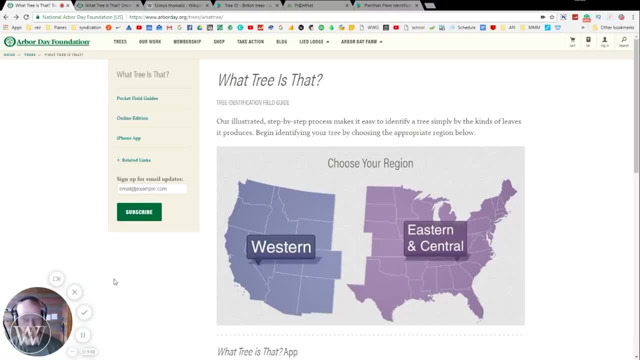 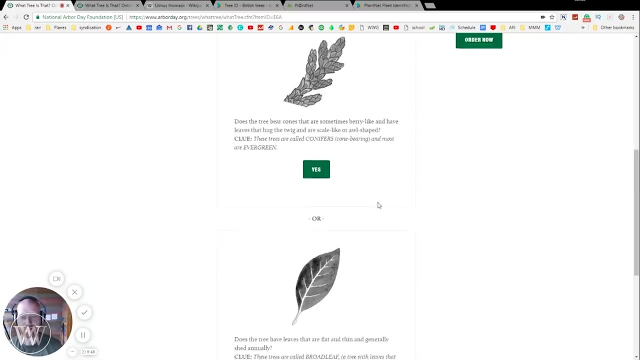 Then you're. this is going to be a little bit more difficult for you, But it's still still fairly doable, because it does have trees that aren't just in North America, Although it is designed for the native trees to North America. So this will basically then go through. you know, is an eastern, is it needles, the cones? is it a regular leaf? 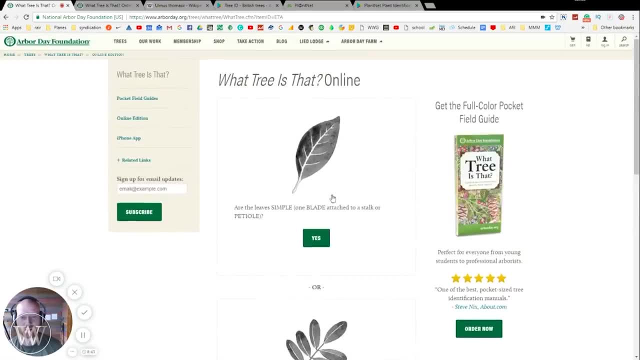 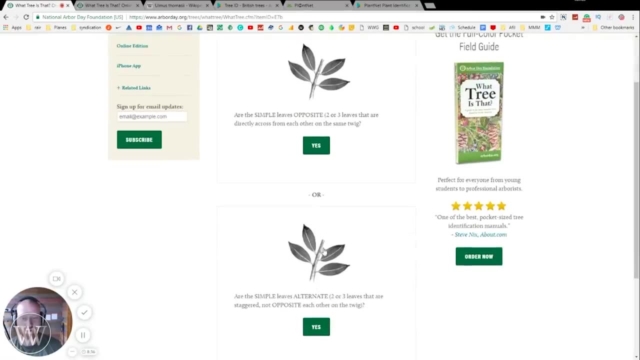 Is it a a standard leaf or is it a compound leaf? You know it's a standard leaf. are the leaves directly across the stem or are they alternating across the stem? and you can go on down through this and it will give you more and more ideas about what it is until 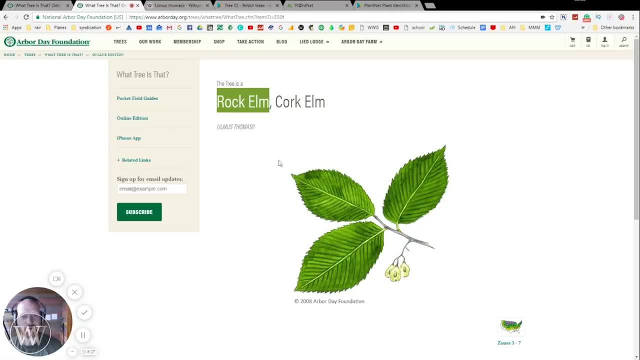 Eventually you come to it. this particular one is a little bit deeper down, So rather than dragging you through that, I'll just take you to the answer. It's an elm tree- I'm particularly a rock elm- and this is a. This is a fairly common one around here. 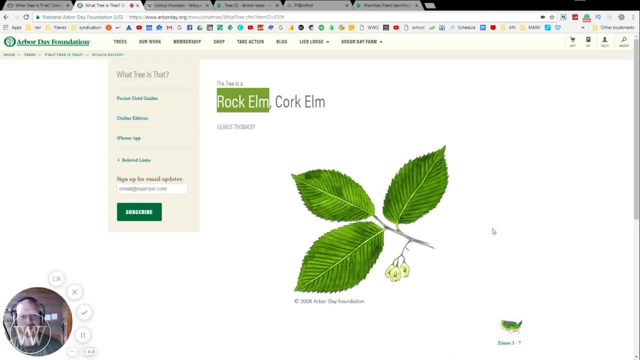 This is actually what my table is going to be made out of, my dining room table to be making here soon. I'm very easily notified by the the paper seeds. You'll find the seed in the middle of the paper And it's a fairly common tree around here. 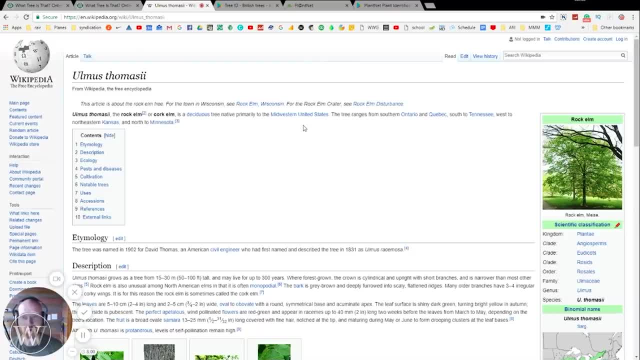 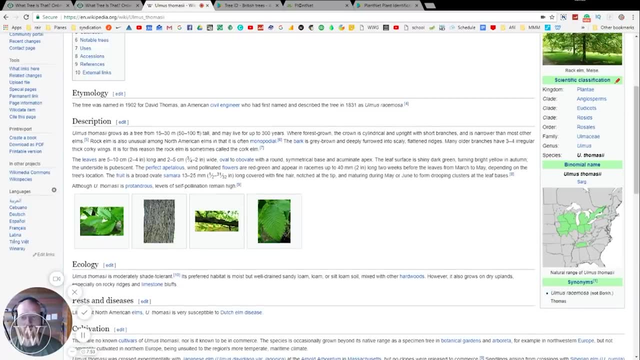 Then the other place that I often go to and I want to find out more information about is wiki. A ton of information on there for you know: more information about what the tree is from history of the name, History about the tree that might be used, different things, far more specifics about where is it located. 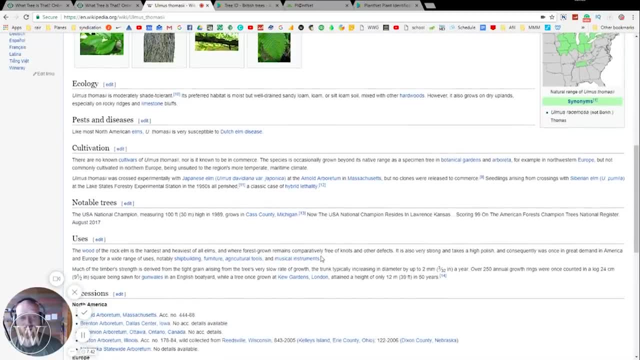 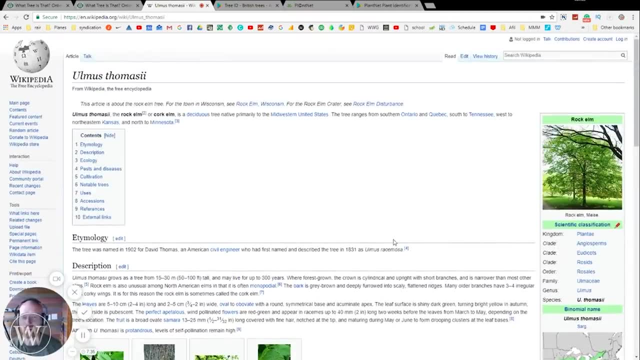 Where is it commonly found, Other uses for it and things like that. This is a wiki, is a great place on Google search in general if you're looking for information Or you kind of know what it is and you're looking for. you know it's an elm tree. 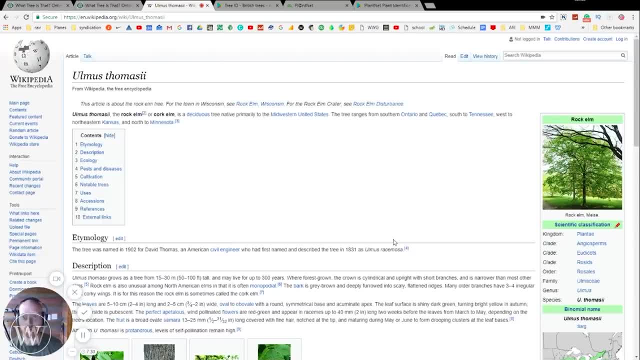 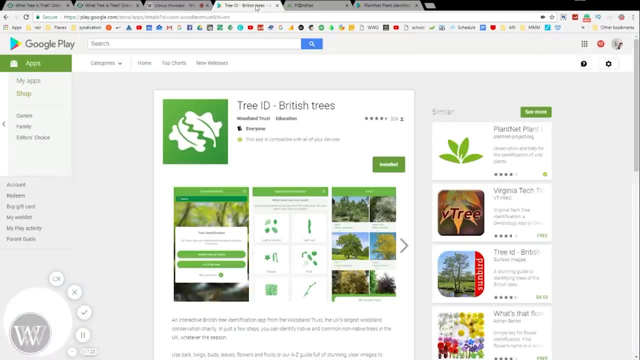 But what type of elm is it? You know, I'll look up elm tree type Leaves and it'll give me pictures of all those and I can kind of match them up and get a better idea from that. Another one that I use all the time is British trees. This is an app you can put on your phone. 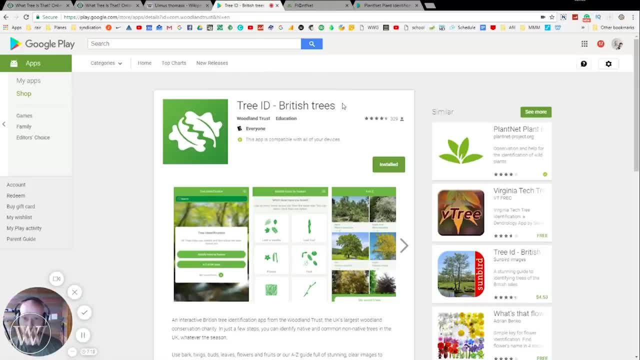 It is focused on trees in Britain, But I'll even find native trees from America listed there, except for they'll be listed as ornamental trees or trees that have been transplanted to the garden as opposed to native trees. and This one is great because it's far easier to get around than the the Arbor Day, because there's pictures. 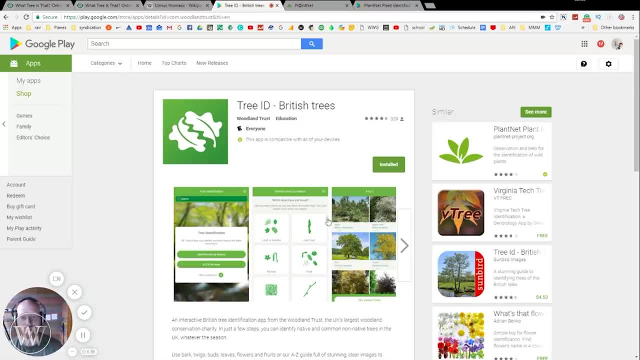 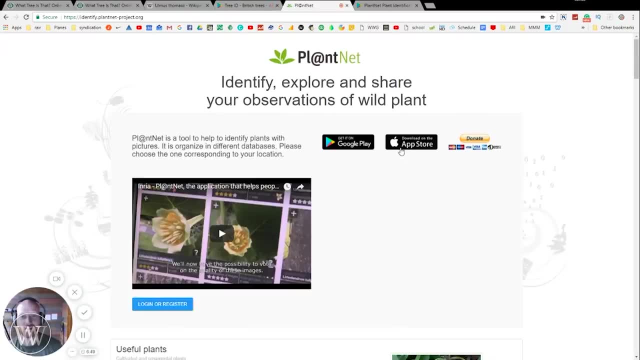 For everything. so if you're trying to find something, this is. this is an app that I use all the time. This is the one I probably use on the fly the most. Then probably the easiest of all of them is plant net with an at symbol in plant. 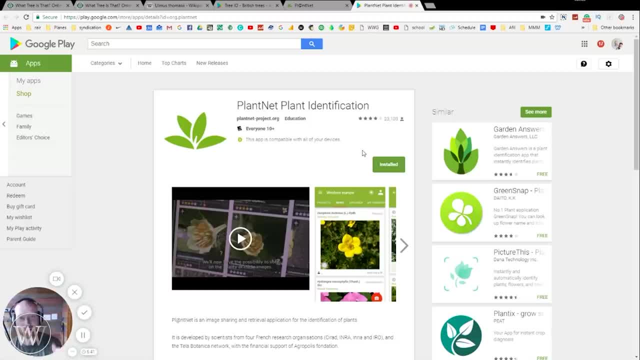 And this one is is so simple because you just take a picture of the tree itself. you take a picture of the leaf or the bud or the fruit and It goes through the algorithm and tries to figure out just from the picture itself. So it's kind of reading the picture. 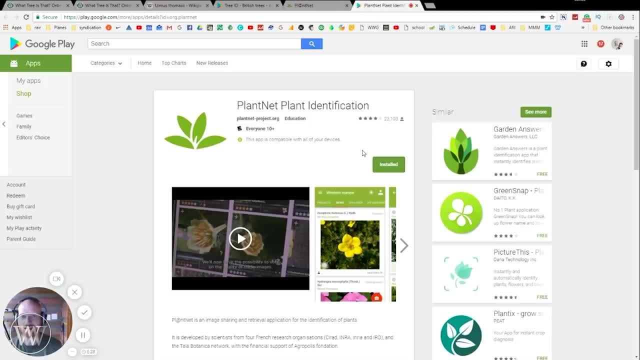 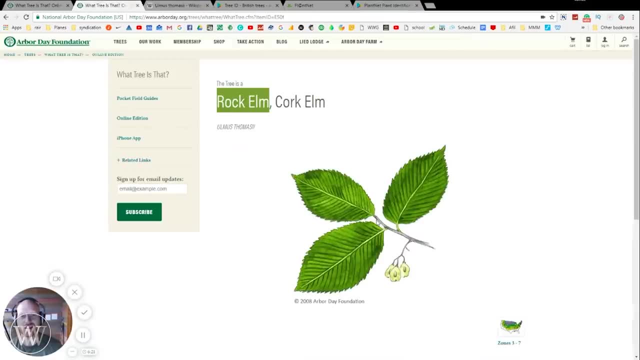 It's very quick, very easy and it gives you a general idea. at least it gives you to a point where you can jump off and you can go and you can google, or you Have more information when you'd go to Arbor Day to to look it up.